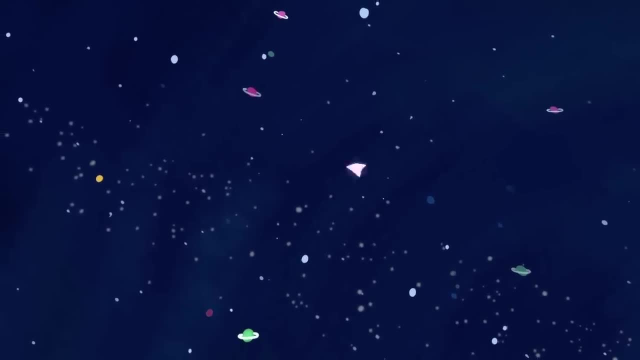 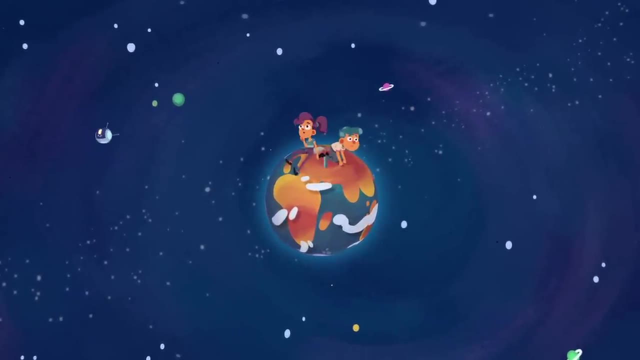 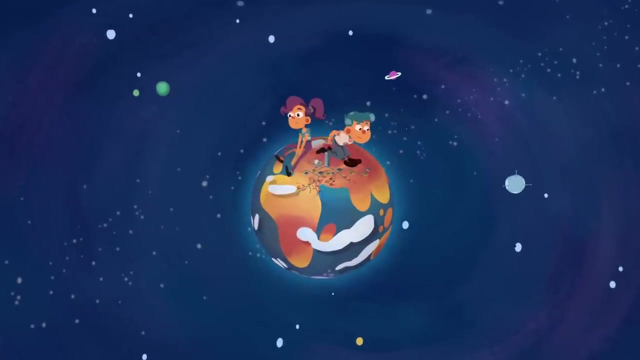 Hi guys, do you have time for a few quick questions? I see you're having a lot of fun, but do you ever stop and think if what you do is sustainable, And do you know what sustainable development means? Sustainable development is to make the world a better place for everyone. now. 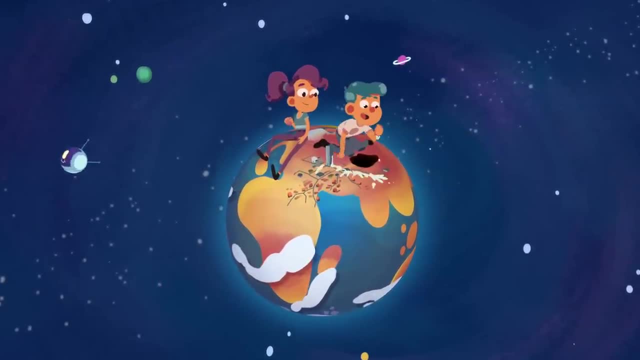 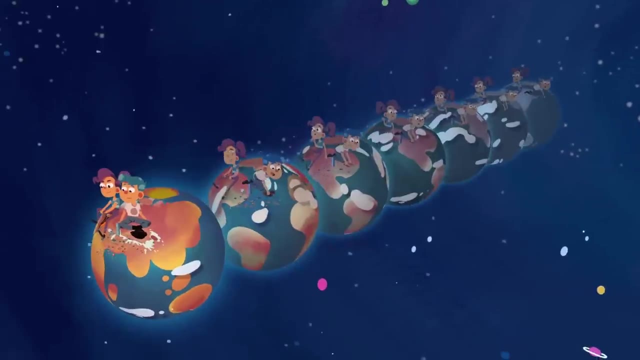 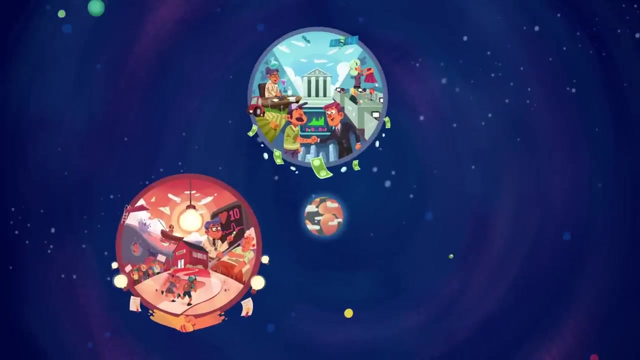 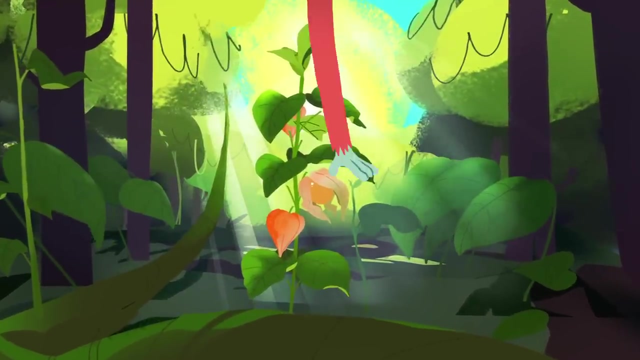 without destroying the possibilities for the next generations. If you wonder if something is sustainable, you can ask yourself: can we do this over and over again forever? Sustainable development means that we need to keep three things in mind at once: Social progress, economic development, and climate and environment. First of all, we have to take care of our planet. 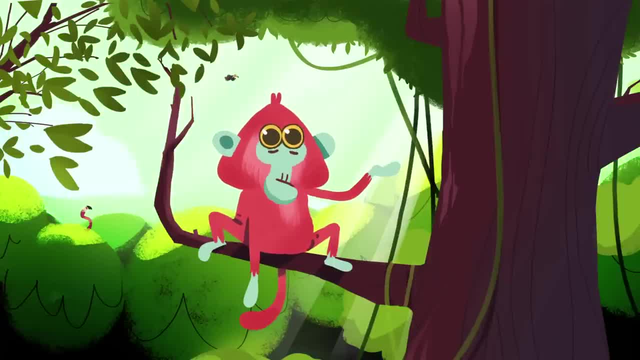 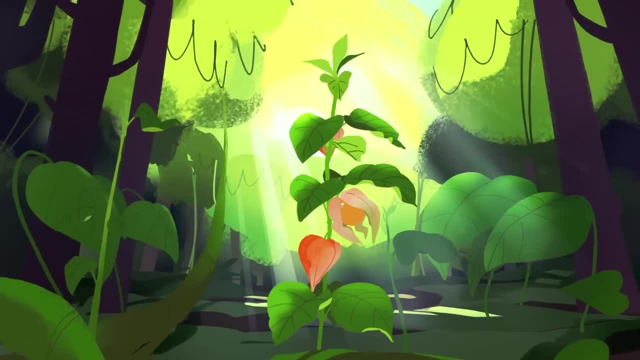 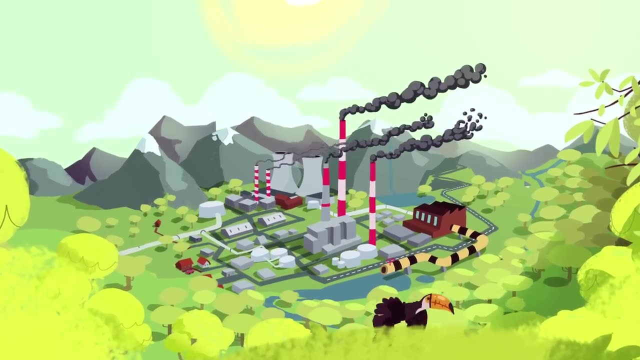 We have many natural ecosystems that must be in balance in order for us to live here. The climate system is one of them. This system ensures that the temperature is correct and that the atmosphere emits exactly the right amount of solar energy When we emit harmful greenhouse gases, such 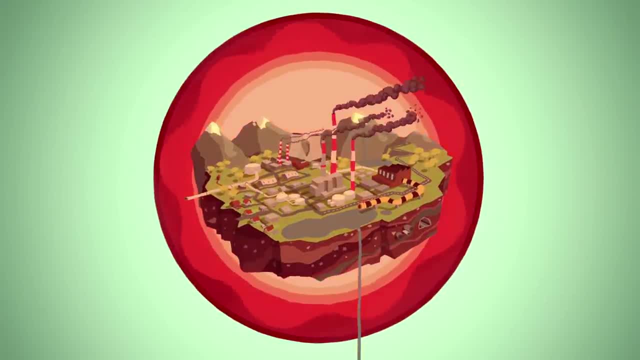 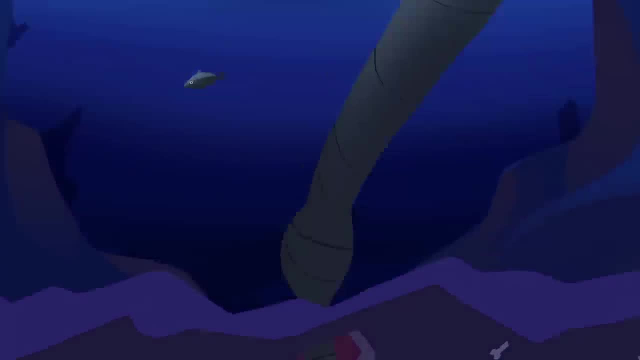 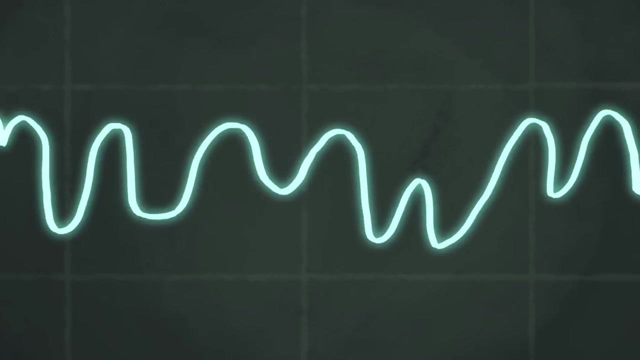 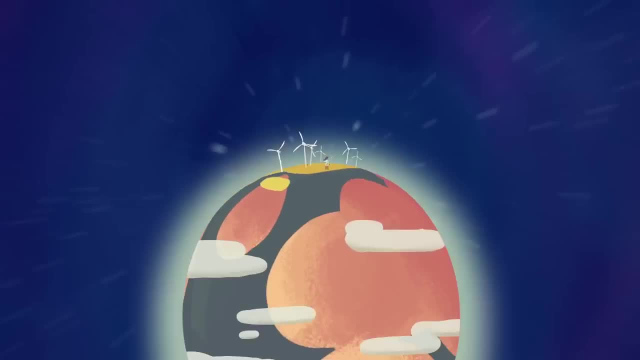 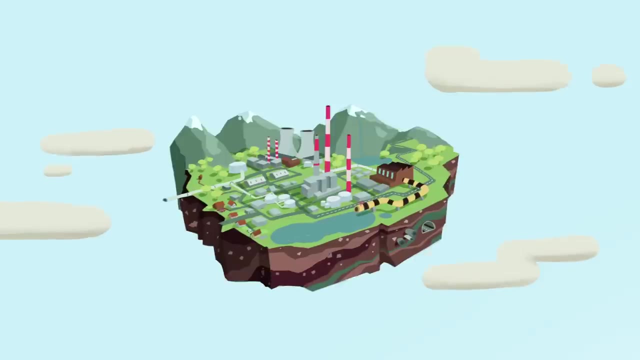 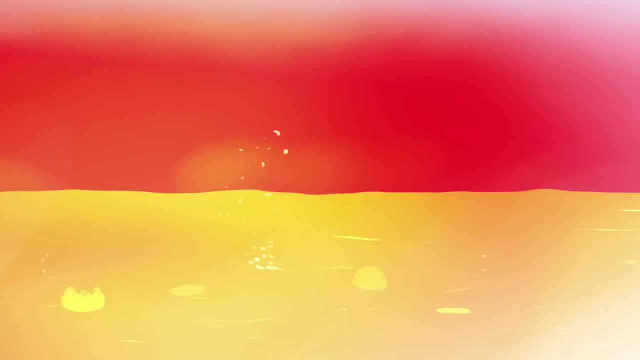 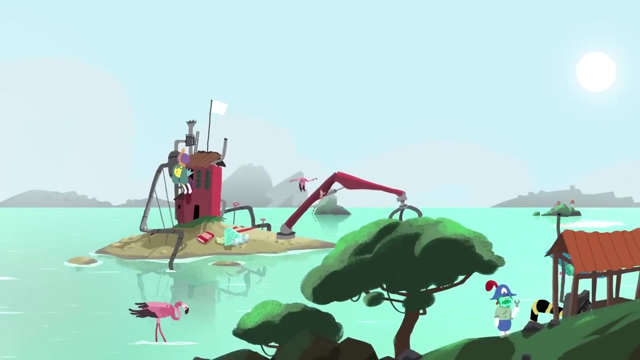 The energy that renews themselves is good for the planet and can provide jobs for years to come. Economics: Almost everything we develop, buy and trade starts with nature. The smarter we use our natural resources and the better systems we create for a fair distribution. 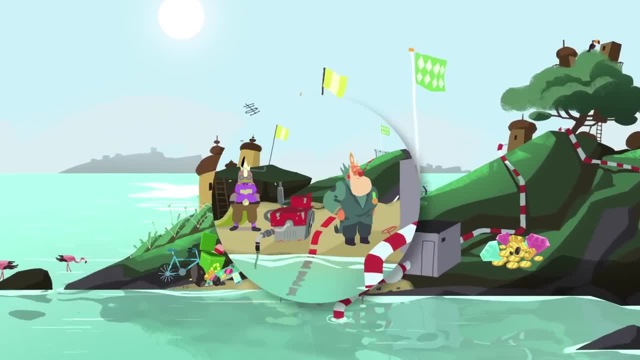 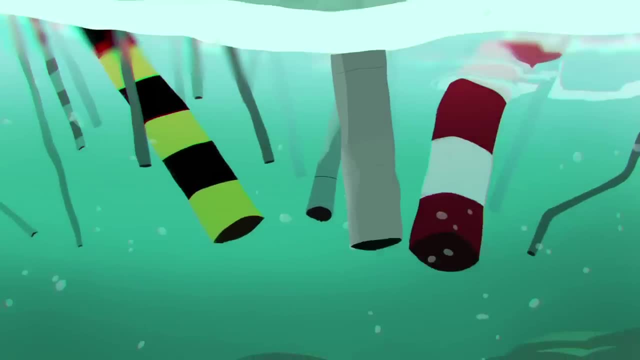 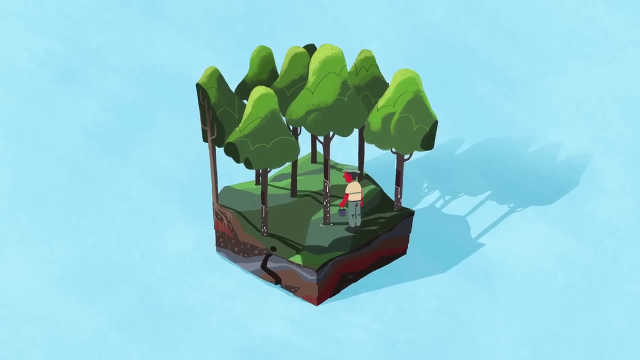 the more sustainable we are. One way to contribute to a more even distribution is to be more aware of what we buy and how it is produced. A football is a good example. It travels far before it reaches the football players. First the materials are made.